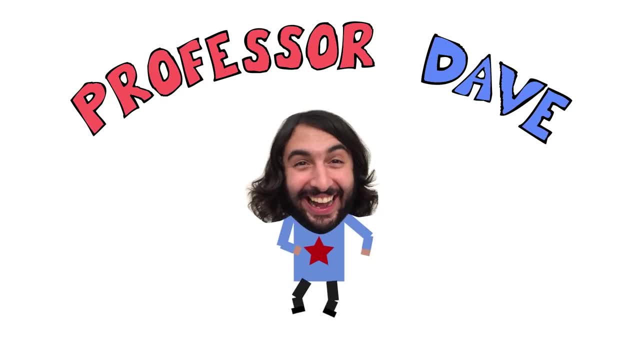 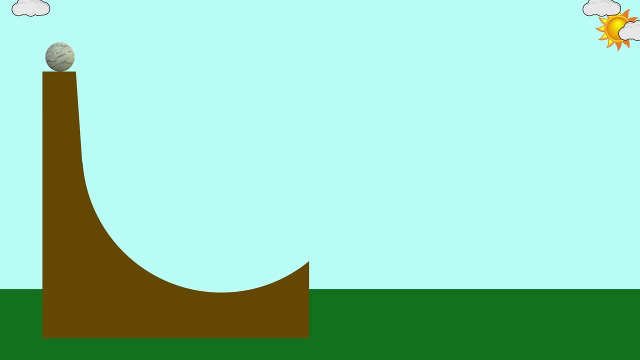 Since you're in the habit of building little bits of physics apparatus at home, you decide to build another ramp, but this one is for a ball to roll down. At the bottom, the track curves back up, launching the ball into the air. 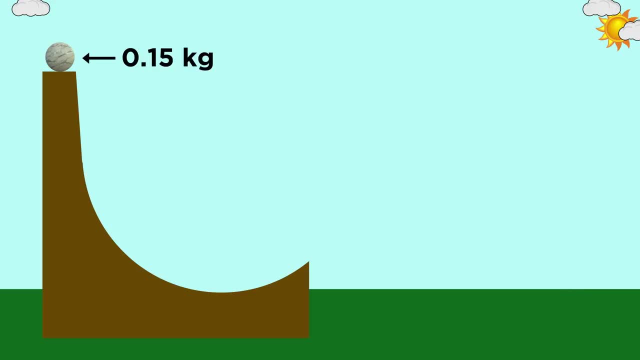 If the ball you use has a mass of 0.15 kilograms and the ramp ranges from three meters off the ground at the top to half a meter off the ground at the lowest point in the path of the ball, what is the velocity of the ball at the lowest point of the ramp and when? 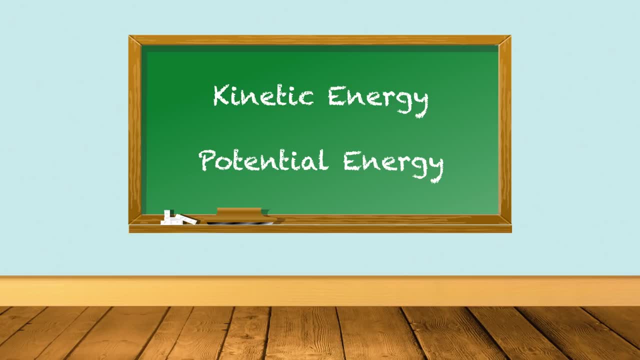 it hits the ground after the jump. To answer this question, we need to know about kinetic and potential energies. so if that sounds unfamiliar, check out my tutorial on this subject in the classical physics series. Otherwise, see if you can figure it out. 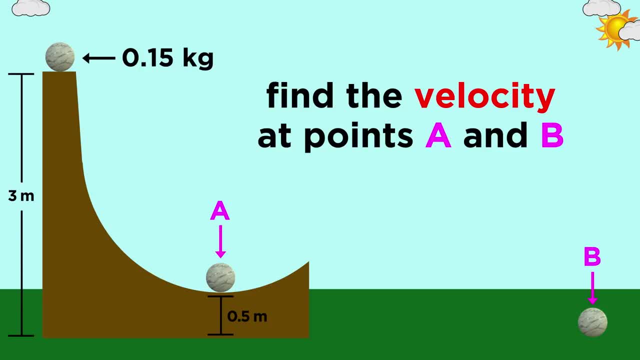 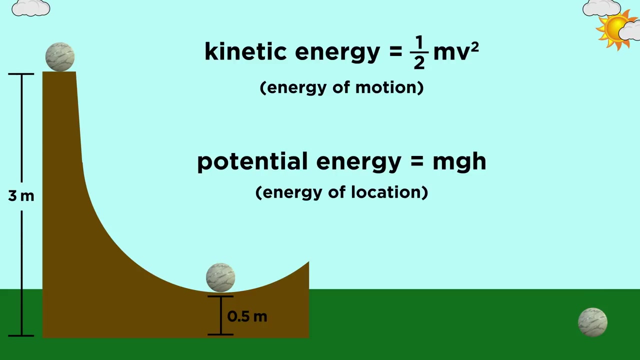 As we said, the name of the game here is kinetic and potential energy. Kinetic energy is the energy of motion And potential energy is the energy of location. At the top of the ramp, before you release the ball, it's not moving, so it has zero. 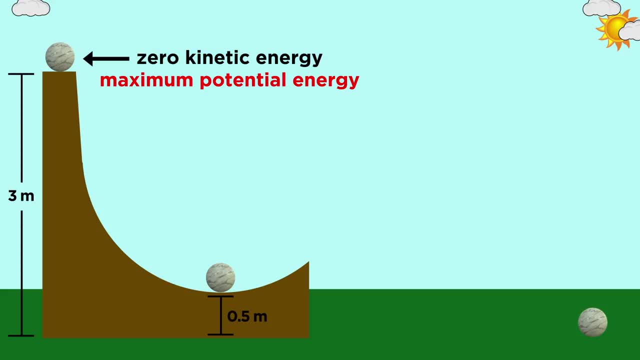 kinetic energy, But it does have some potential energy. To find out exactly how much we use the equation, We can plug in the mass acceleration due to gravity and the height of the ramp and we get 4.4 kilograms meters squared per second squared, or 4.4 joules. 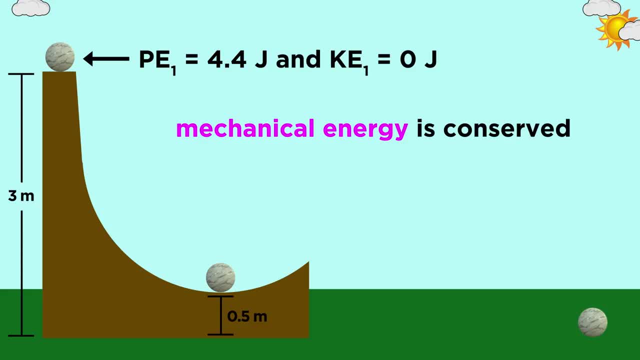 Now what we also have to understand is that as the ball moves down the ramp, the total mechanical energy is always conserved, meaning the sum of the kinetic and potential energies- in this case 4.4 joules- is constant. So as the ball gets closer to the ground, potential energy is being converted into kinetic. 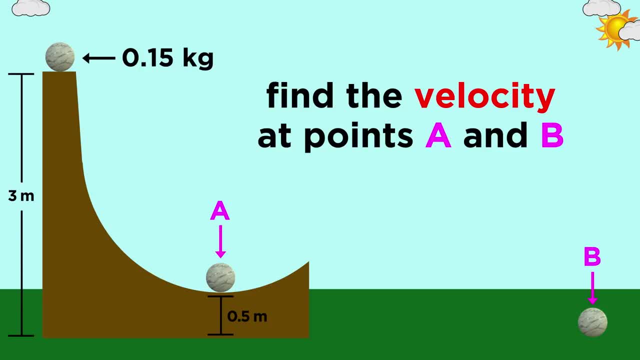 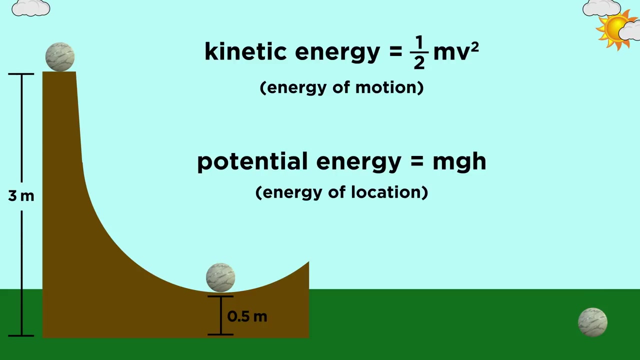 As we said, the name of the game here is kinetic and potential energy. Kinetic energy is the energy of motion And potential energy is the energy of location. At the top of the ramp, before you release the ball, it's not moving, so it has zero. 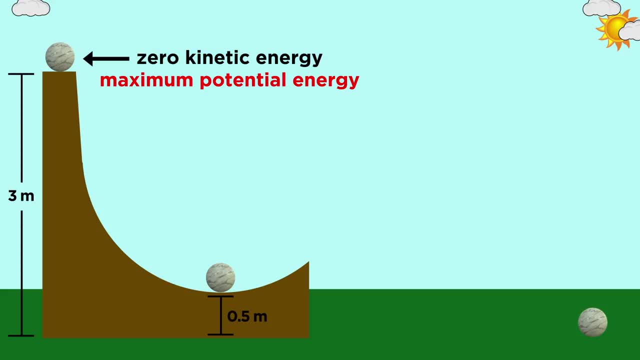 kinetic energy, But it does have some potential energy. To find out exactly how much we use the equation, We can plug in the mass acceleration due to gravity and the height of the ramp and we get 4.4 kilograms meters squared per second squared, or 4.4 joules. 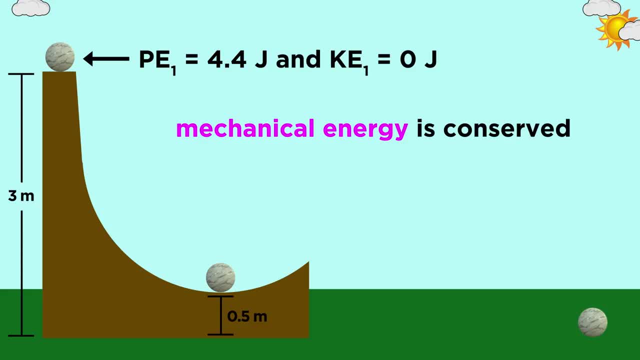 Now what we also have to understand is that as the ball moves down the ramp, the total mechanical energy is always conserved, meaning the sum of the kinetic and potential energies- in this case 4.4 joules- is constant. So as the ball gets closer to the ground, potential energy is being converted into kinetic. 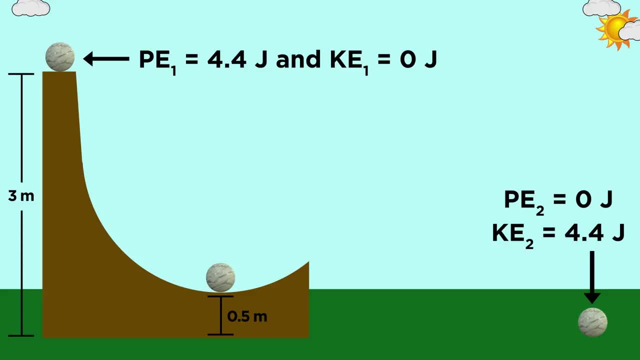 energy. That also means that the instant the ball hits the ground where it has zero potential energy, it must have converted all of its potential energy into kinetic energy. so the kinetic energy of the ball at that moment must also be 4.4 joules. 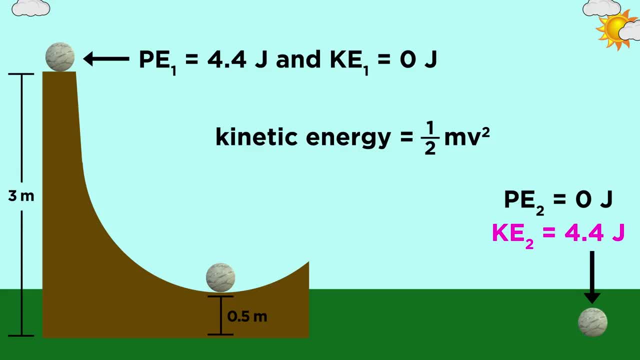 Now we can use that to find the velocity of the ball at the moment of impact: 4.4 kilograms meters squared per seconds squared is equal to one half the mass times velocity squared. so we simplify a bit. Take the square root and 7.66 meters per second is what we get. 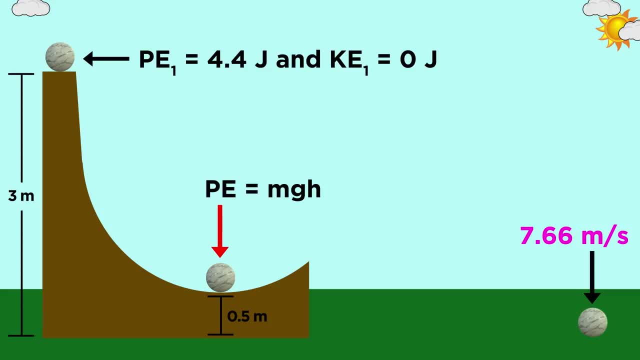 Now for the lowest point of the ramp. Let's get the potential energy first, which will be the same mass and acceleration as before, but the height is now half a meter. That gives us a potential energy of 0.74 joules. 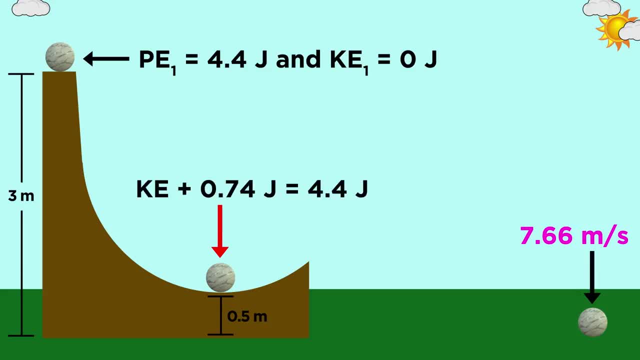 Kinetic and potential energies must add up to 4.4 joules. so the kinetic energy at this moment must be 3.7 joules. With that we just plug into the same equation as before, rearrange and take the square.